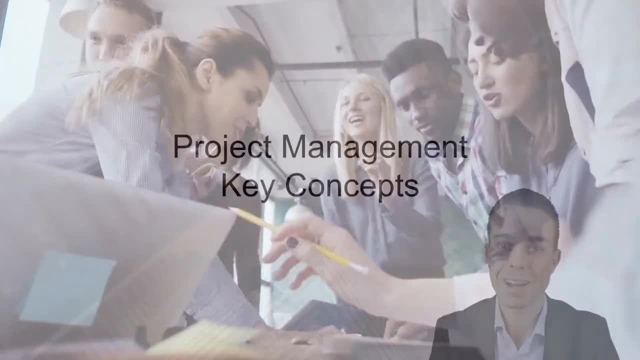 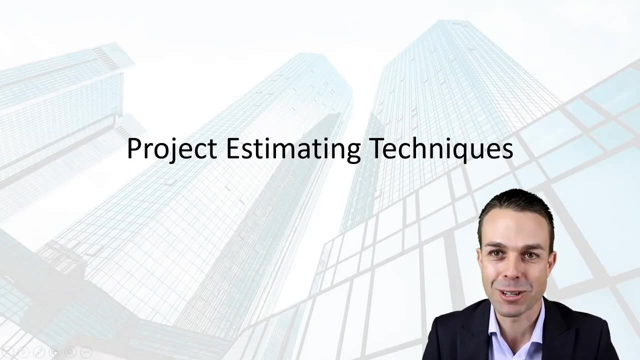 Hi everyone, welcome back to this series of project management key concepts where we're delving deeper into the project management body of knowledge. This one in particular is project estimating techniques. Now, you will definitely see these mentioned as part of the PMP exam, so it's good to know that there are four main different types and the differences. 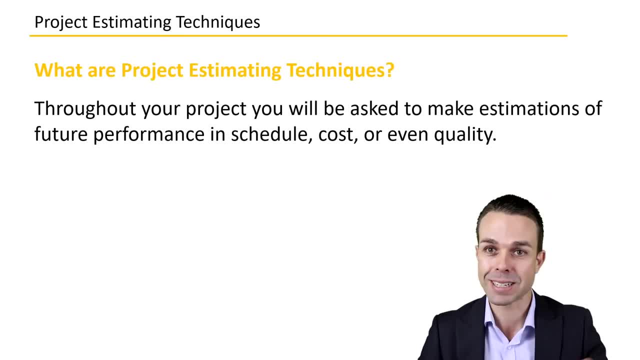 between those types. So what are project estimating techniques? Well, throughout your project you'll be asked to make those estimations of future performance, and that could be in your schedule, could be in the cost of the project, it could even be in the quality of your project. But the 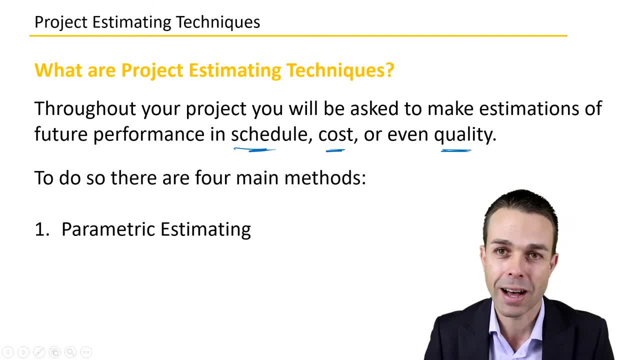 four main methods that you will come across as part of the PMBOK guide are parametric estimating, bottom-up estimating, analogous estimating and three-point estimating. Now they might sound a little bit funny, but we'll go into them in a little bit more detail. First of all, we've got 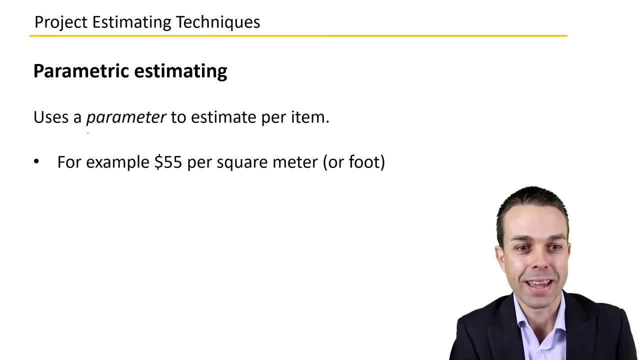 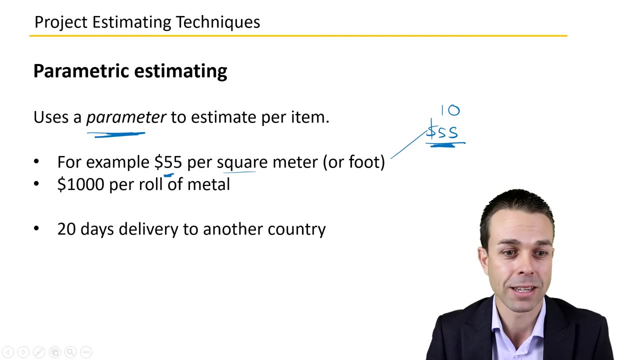 parametric estimating. This is where we're actually using a parameter to estimate per item, So it's a simple parameter. let's say $55 per square meter or square foot. We might have $1,000 per roll of metal or whatever. that is 20 days delivery, for example, in our schedule that it might take to get to another. 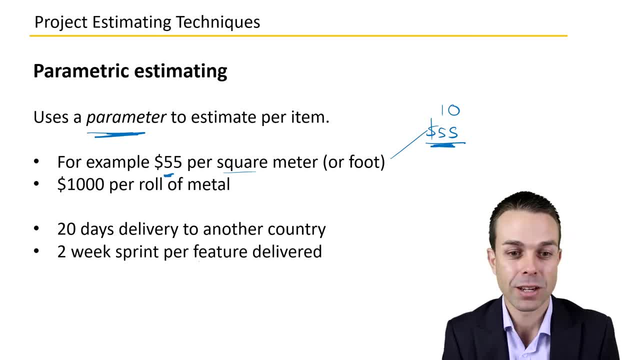 country, Or we might be looking at two-week sprints per each feature that we're delivering in a software project. A team might take an eight-hour workday to get to another country, or we might be looking at two-week sprints per each feature that we're delivering in a software project. 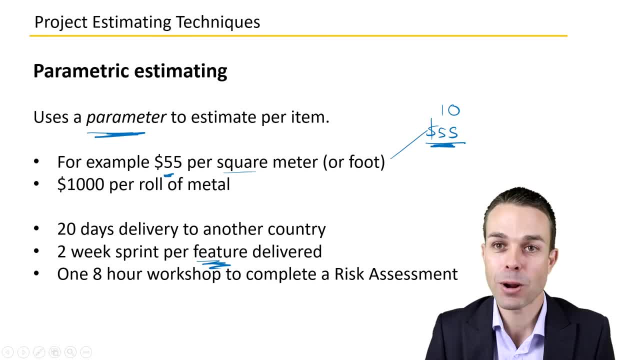 Or we might be looking at two-week sprints per each feature that we're delivering in a software project, Or we might be looking at two-week sprints per each feature that we're delivering in a software project. So all of these are parameters that we might assign to the activities so that we can estimate for. 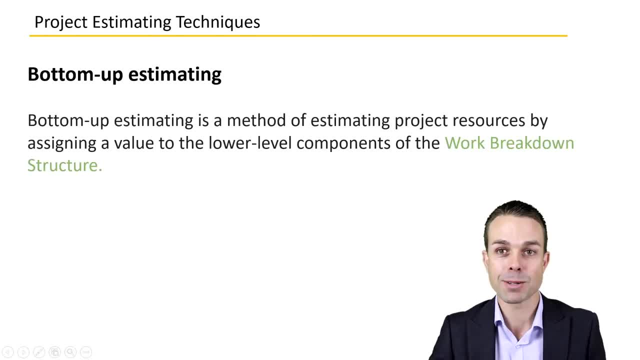 those activities Next up. we've got bottom-up estimating. Now this is where we're estimating project resources by assigning a value to the lower-level components of the work breakdown structure. We're starting from the bottom and we're working our way up, And when we say the 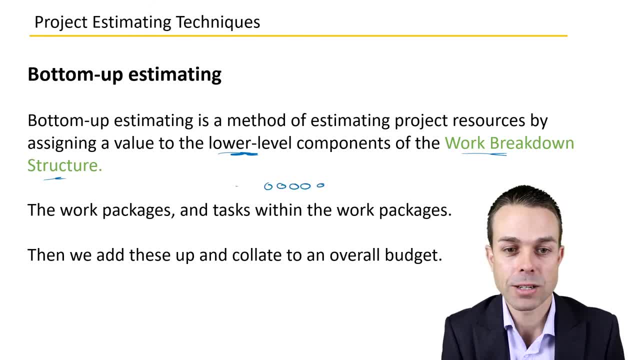 bottom we mean the lower-level tasks that have been assigned to our teams. Now these, of course, go up in the work breakdown structure to larger tasks or features and then to an overall delivered feature, for example- And this is where we start getting into agile potentially- or feature-driven. 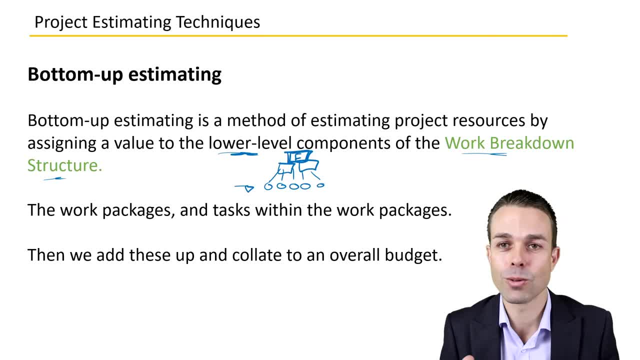 development. But all of those things are interrelated. They're all ways of working that are across disciplines. But the idea of that is that we will assign this team can estimate on their piece of work. this team can estimate on their piece of work or their single task or one. 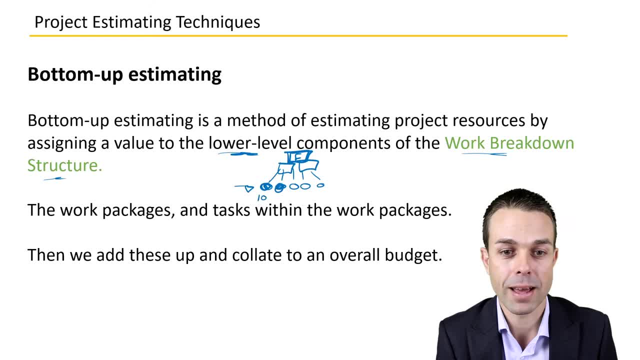 or two tasks And that might be, let's say, $10,000.. This one might be $20,000.. This one might be $5,000.. And then we take all of those items and we bring them up into the feature. So 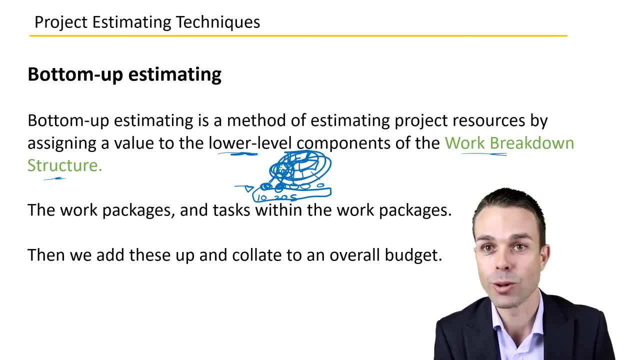 the total there could be 50. And then the total for the overall feature could be $100,000,, for example. But the key is that we're starting at the very lowest level of the activity. We're starting from the bottom Next up. we have analogous estimating. Now this is where we're finding. 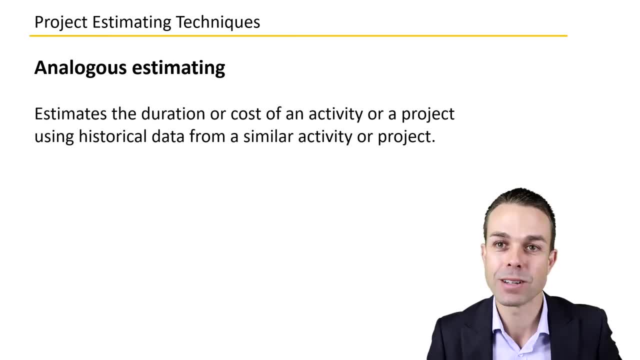 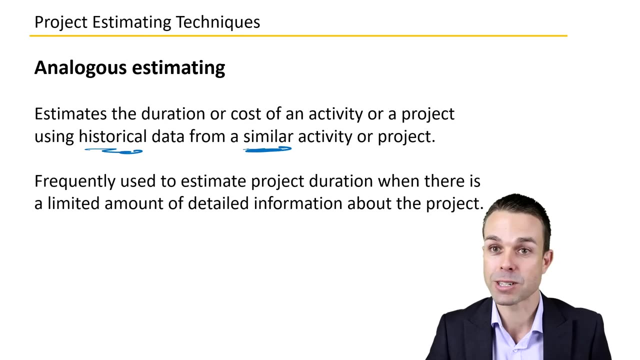 an analogy, Something similar to what we're currently doing. So we're estimating the duration or cost of an activity or a project using historical data from a similar activity or a similar project. Now, of course, this is frequently used to estimate project duration when there is a limited amount. 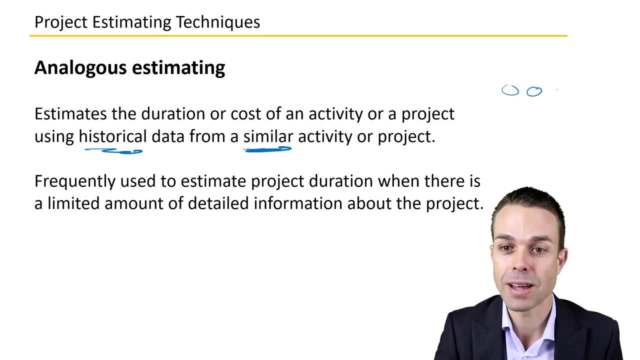 of detailed information. So we haven't gotten down into the work breakdown structure yet at the team level We only have a really high level idea. Maybe we can get a rough idea of how this is going to work. So we're estimating the duration or cost of an activity or a project. 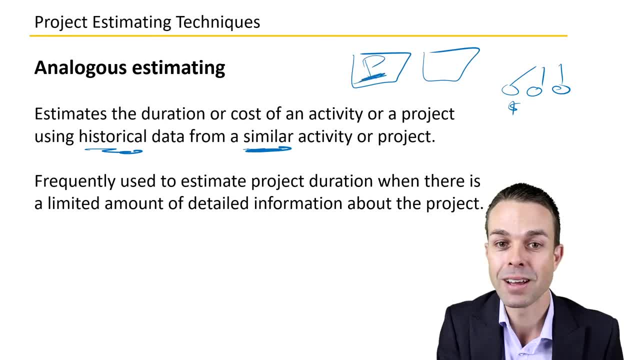 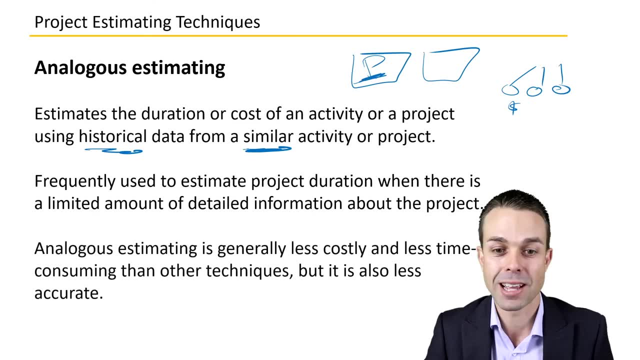 Much it will cost or how long it will take by looking at another similar project. It's like an analogy. It's similar to what we're currently doing Now. generally it's less costly and less time consuming than our other techniques, but also it is less accurate because we're not really 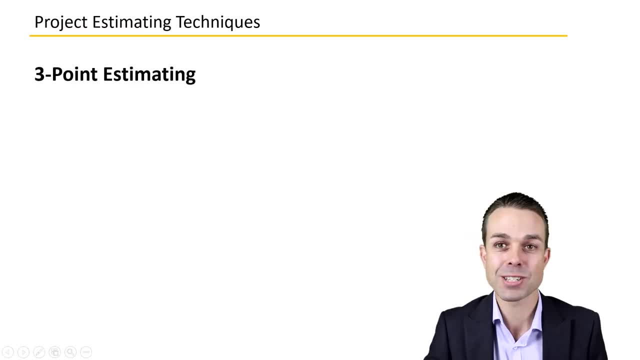 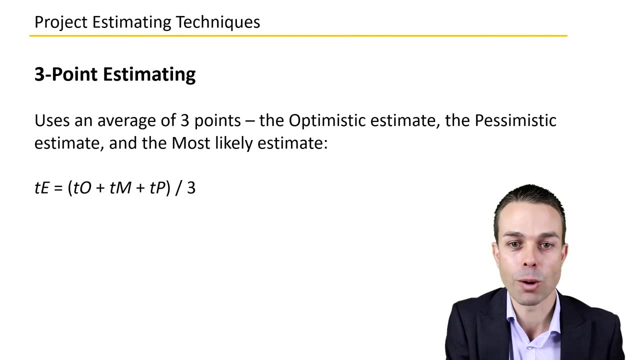 delving into the detail. Now, last but not least, there is three point estimating that you will come across. This uses an average of three points. We might have the optimistic estimate, the pessimistic estimate and the most likely estimate And the way that we end up working it. 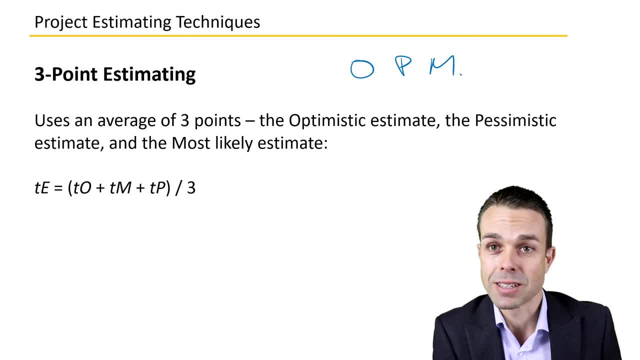 out is the optimistic. Let's say, our optimistic schedule, for example, is five days, Our most likely is seven days, And then our pessimistic is 10 days, And then we divide that by three And that gives us our answer. In fact, I've got a better version of that that doesn't take as